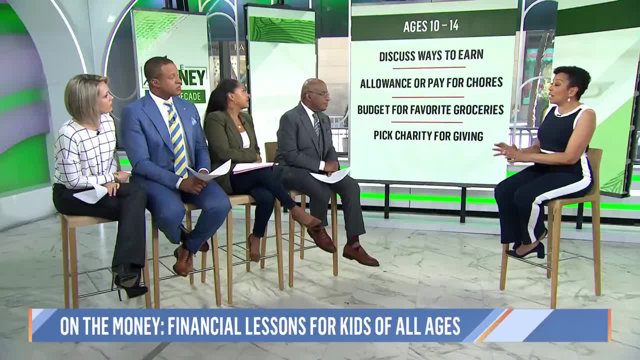 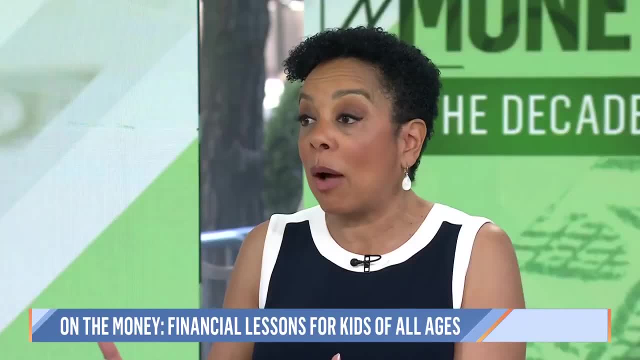 start understanding budgeting. Yeah, I think it's important to understand budgeting, but also that it takes income to budget. right, There you go. You have to discuss with them ways that they can earn. Maybe you're going to give them an allowance for certain things that they're doing. pay them. 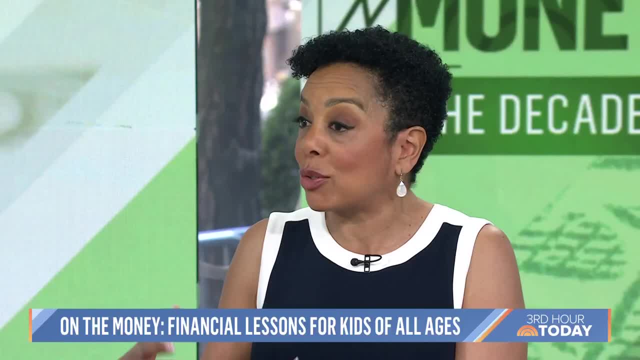 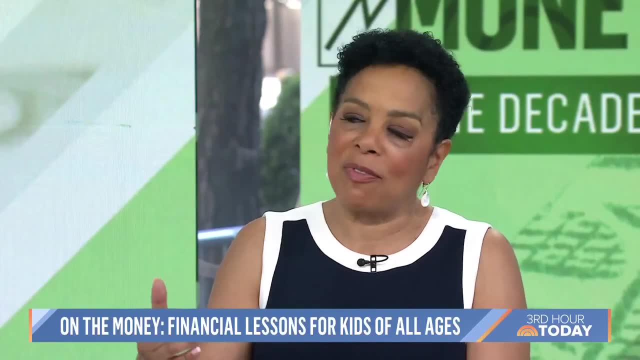 for chores that they may do around the house. I think that's very important to make sure they understand that they're working for something and that's how they're being reciprocated. But when I talk about budgeting, maybe you have some favorite items that you know your child loves You go to. 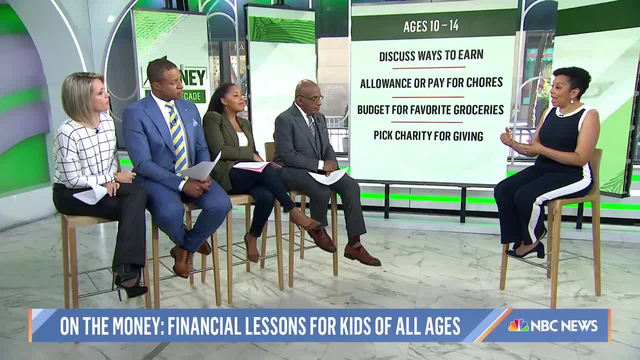 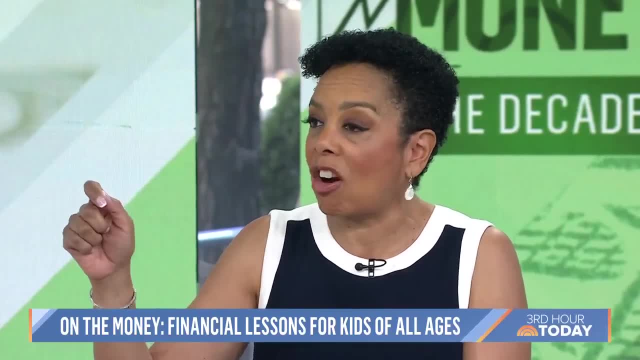 the grocery store together. give them a budget to buy those things- And these are things you love, but this, this is all the money that you have. Once that's gone, you can't get anything else. Don't say you put this in the cart. The other thing that I loved doing with my kids when they 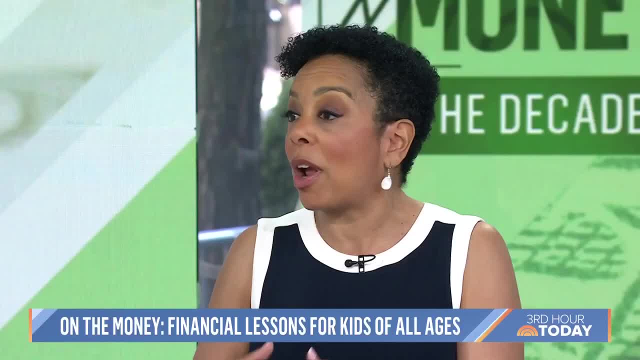 were that age was picking a charity with them. Where do they go Where? what charities are in your community that you want to support? And it doesn't always have to be with money. It can be with them learning how to donate clothes or spending time with people. So that's something. 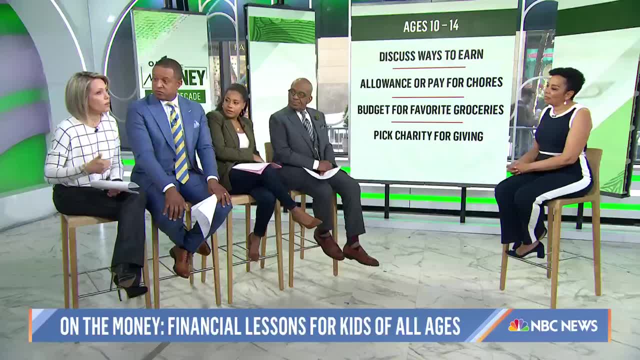 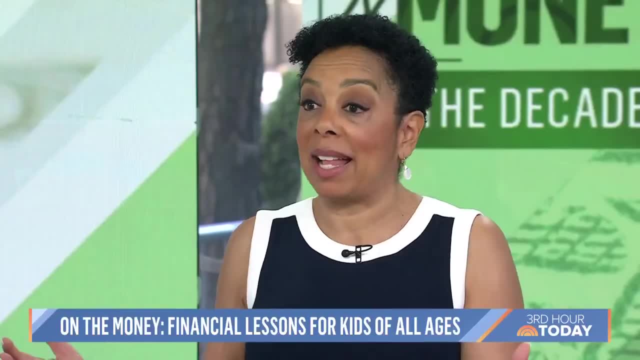 really important to foster that. early In high school I worked. I saved money, but I wish I learned how to invest money. Why is that important? Because we love brands. Kids love brands, Adults love brands. but we need to understand. we want to buy the company that makes. 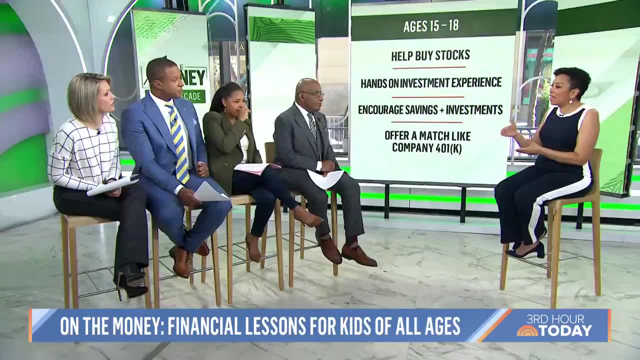 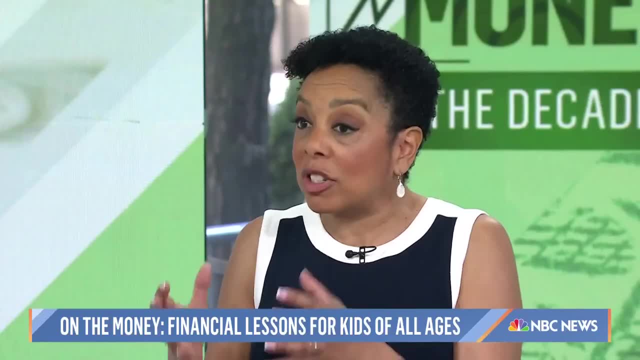 those brands And so teaching them to love having a stake in the game with that company so important. You can set up investment accounts. There are apps that can help you. You can do it online: setting up an account and teaching them that giving that the hands-on experience is. 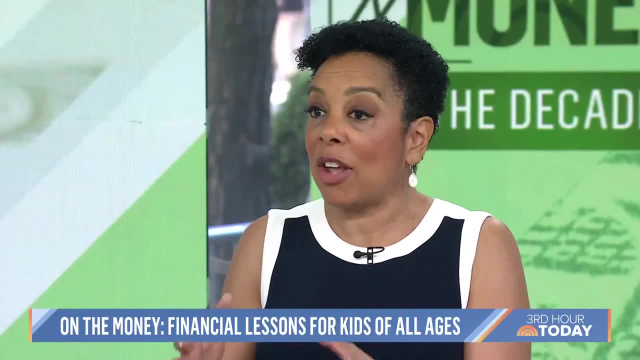 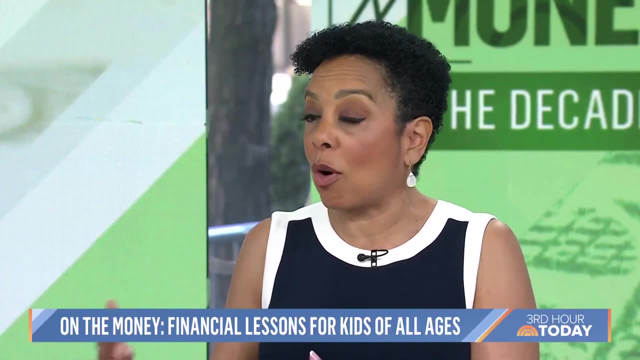 important, but also understanding that you have to save- and you have to save for a rainy day- and encouraging them to save some of their own money, whether it's gifts that they get at for a birthday or for a holiday. maybe you match that Like we get to a 401k match. People love when their 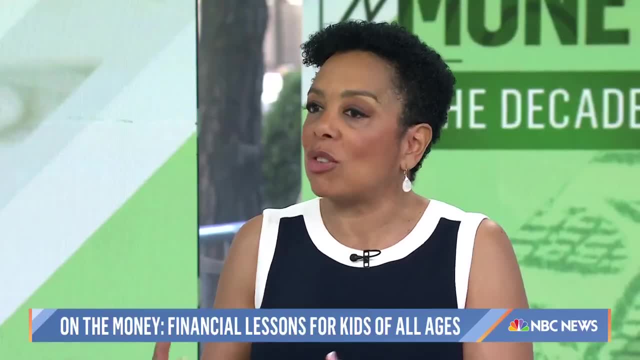 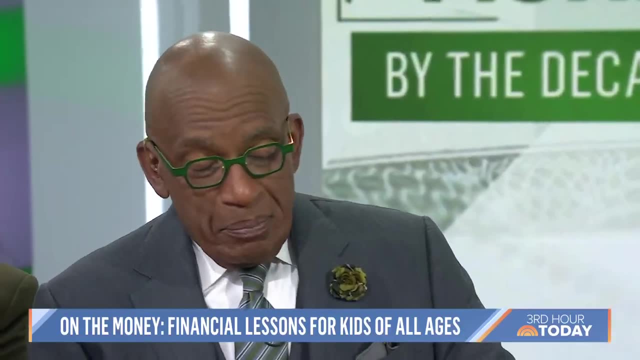 employers do that. Maybe you match it for them to kind of also help them. It's a great idea. We're just finishing up next freshman year of college And one of the bumps has been we probably didn't prep them or ourselves, for our kids going off on their own. 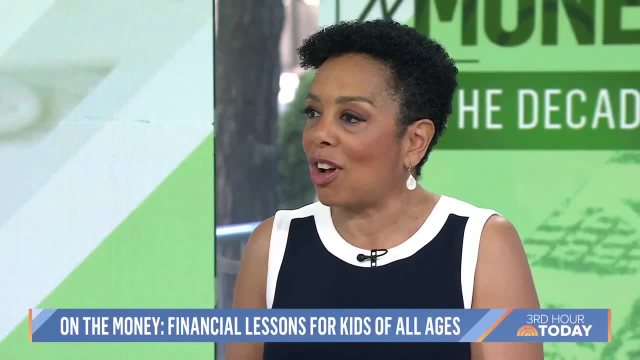 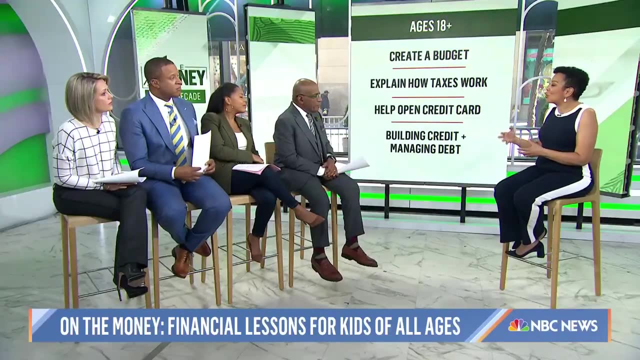 and budgeting that money. I'm right there with you- And it's such a difficult conversation to have- and the way that they spend, because they're just used to doing it. Sometimes, if they don't have a budget, they just keep spending, So creating that budget is very important early on.